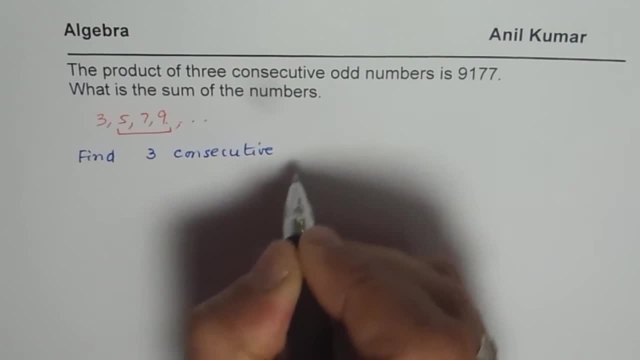 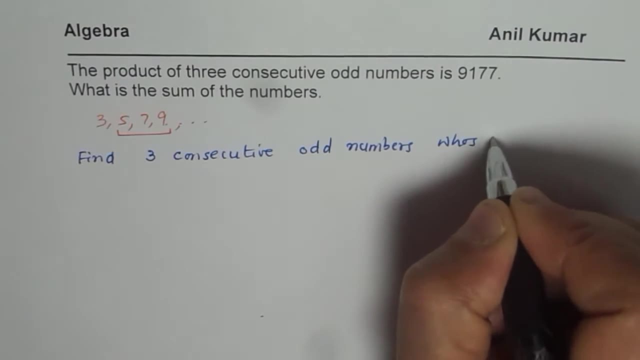 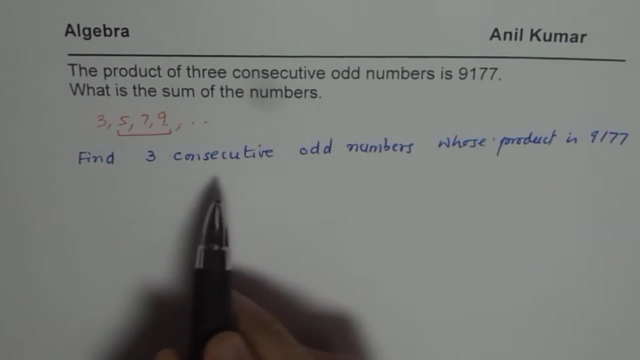 odd numbers whose product is 9177. And then, once you find, you add them up and then you get the answer for the second part. Now, how to get those numbers. There are different strategies which you can work with. One is kind of you can estimate, But I think the 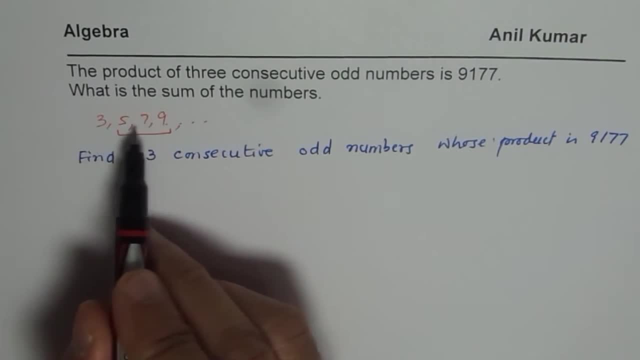 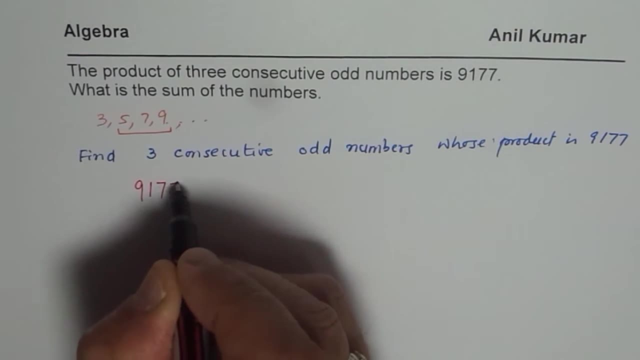 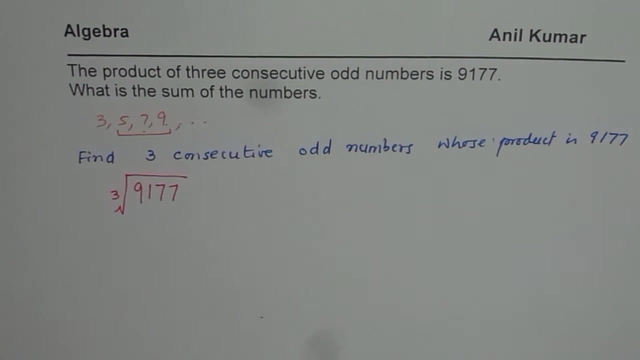 best strategy is if we are multiplying three numbers like that which come together, if I take cube root of the number, then what happens? So 9177,. if I do cube root of this, then I get the number in the center right of that series. So let's do that, So we have. 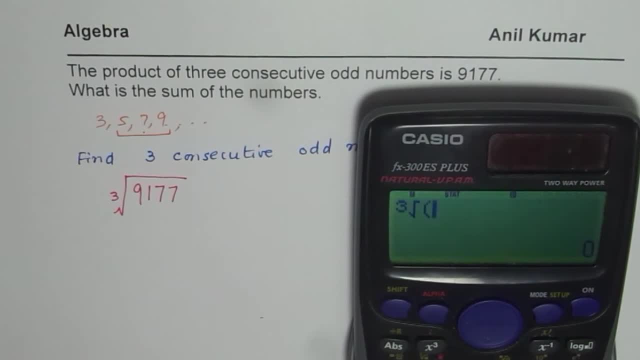 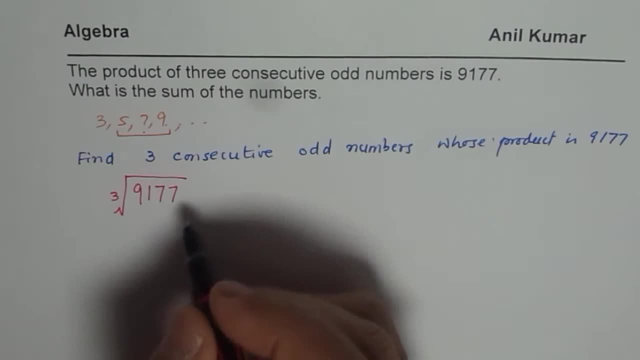 cube root. and here we have shift cube root and the number is 9177.. Cube root is 20.93.. So cube root of this is equals to 20.93.. So that gives me kind of idea, right. So the center number is close to 20.93.. Of course, the odd number, which is very close to this. 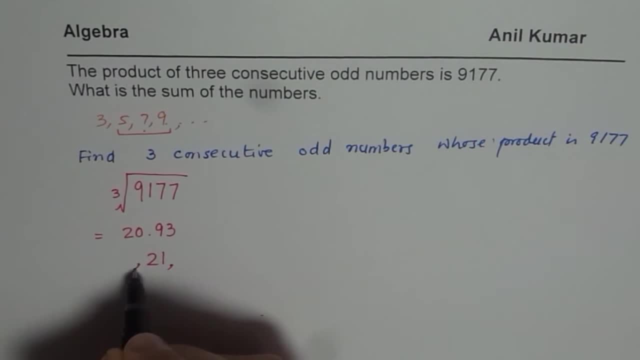 is 21,. right, So 21 is one of my numbers. The other two numbers are before and after. Odd number which comes before 21 is 19 and the one which comes after 21 is 23.. So that's it. 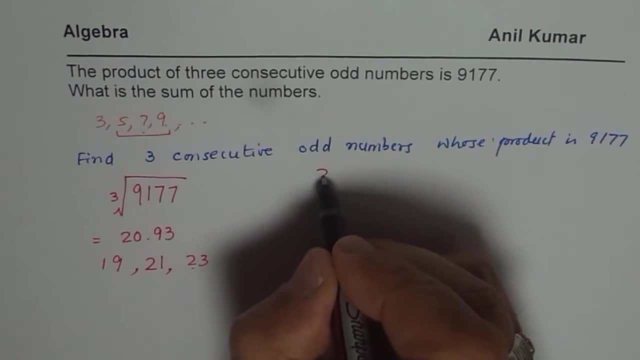 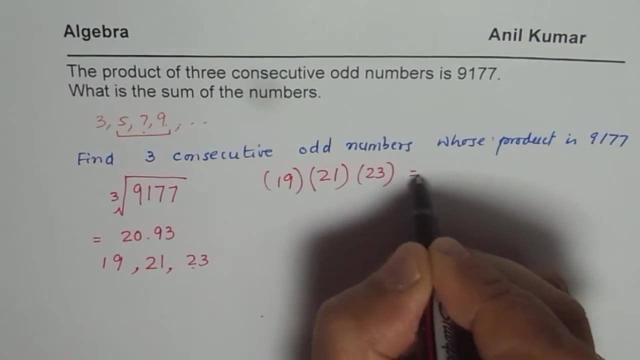 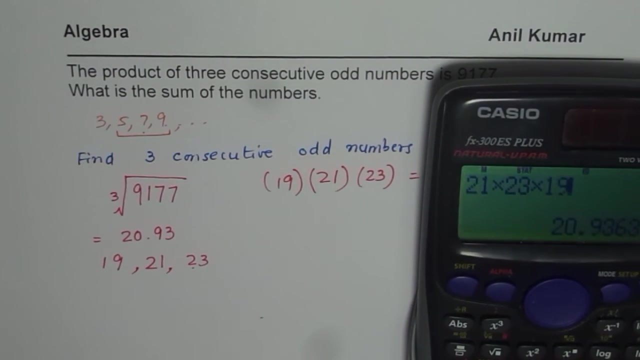 So that could be my solution. So let us check. So let us check with 21 times 19 times 23 and see what do we get right. So what we will do is we will multiply 21 by 23 and 19.. 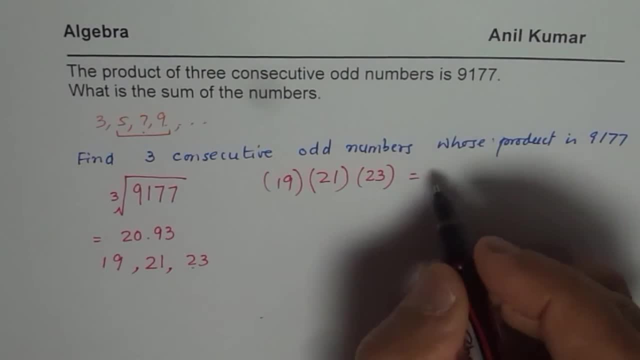 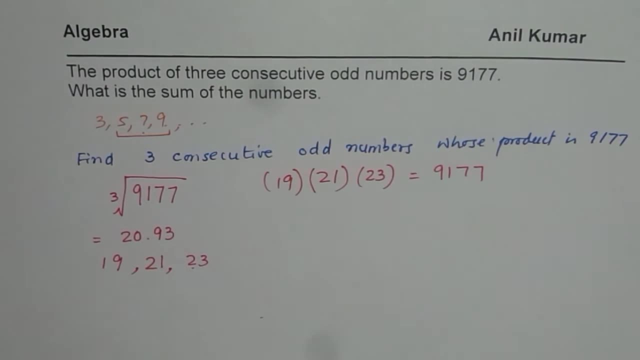 We get 9177.. So that is perfect. So we get 9177.. So these are the three consecutive odd numbers whose product is 9177.. Now the next part is to find some of these numbers. So what is their sum? So sum is you. 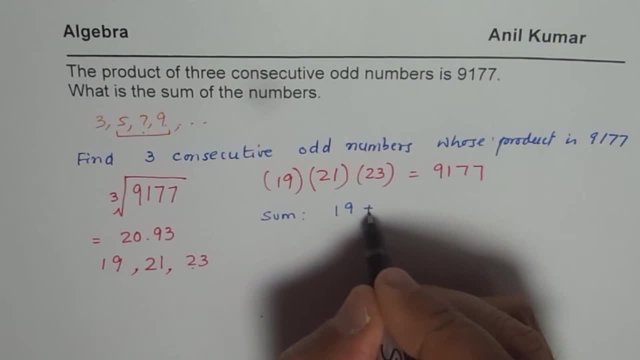 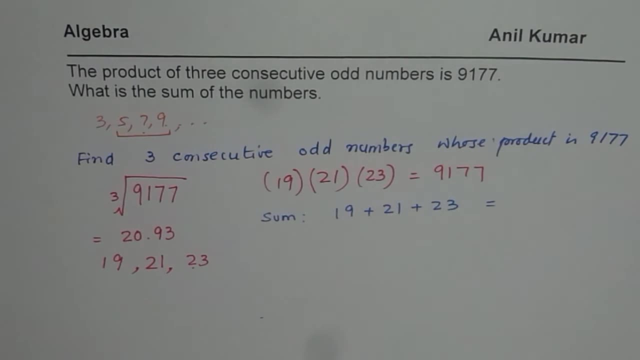 can just add them up, right, So you do 19 plus 21 plus 23,, correct, and get the answer. So that is the answer, which is three times the middle number, correct? So three times the middle number could be 63.. So that is how we can do it, or you can just add them.